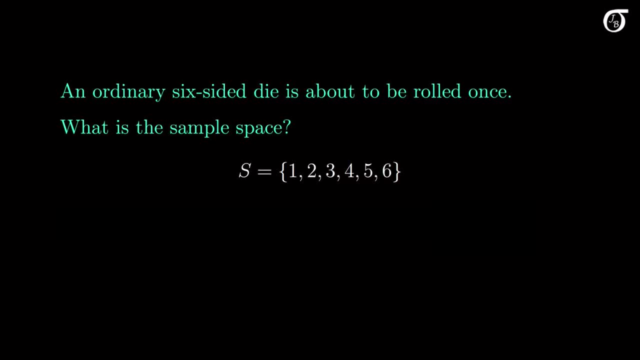 But in this situation it's quite natural to have the sample space contain the six possible numbers that we can roll. What is the probability that a 2 is rolled when we roll the die once Here it's reasonable to think that the six sample points are equally likely. 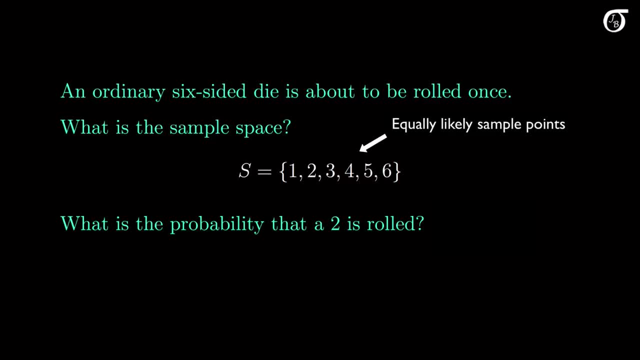 As long as it's an ordinary die and we're rolling it fairly, then that's a reasonable assumption to make, Since exactly the same number of points are equally likely and only one of the six equally likely sample points is a 2,. 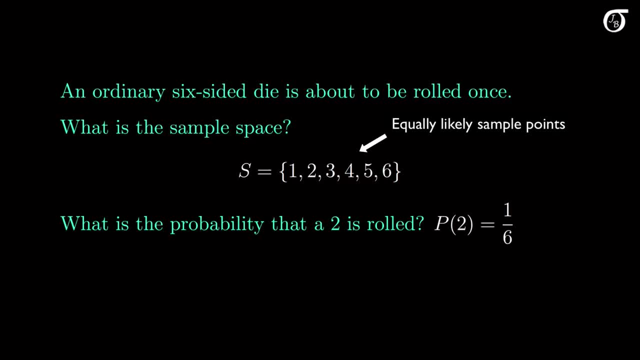 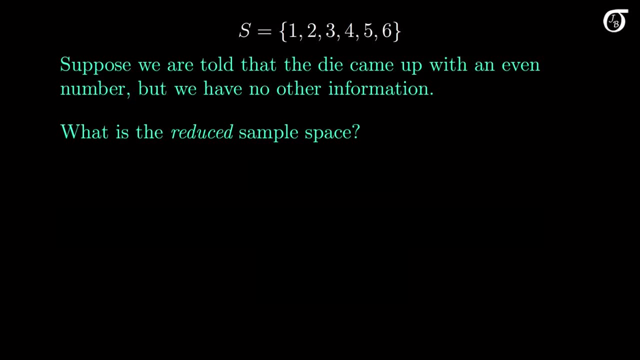 the probability of rolling a 2 is 1 out of 6.. Here's a slightly different scenario. Suppose we are told that the die came up with an even number, but we have no other information. What is the reduced sample space? We know that the number is even, so 1,, 3, and 5 can't have occurred. 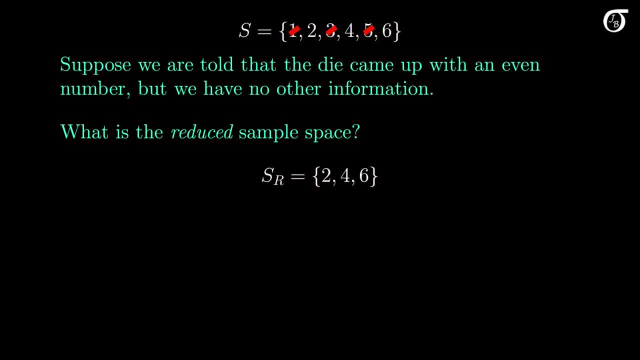 The reduced sample space is now the even numbers. Suppose we were asked the question: given an even number is rolled, what is the probability it is a 2? Here we are looking for a conditional probability, the probability that we rolled a 2, if we know the number is even. 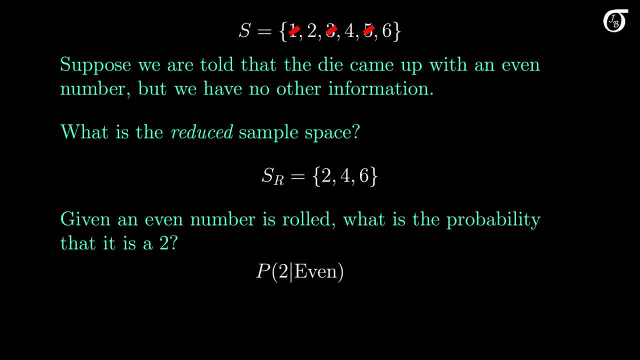 Notation-wise, we might write that as the probability of 2, given even where what comes after the vertical bar is known to be true or assumed to be true for the purposes of the question. Now, in a moment we are going to look at the official definition of conditional probability. 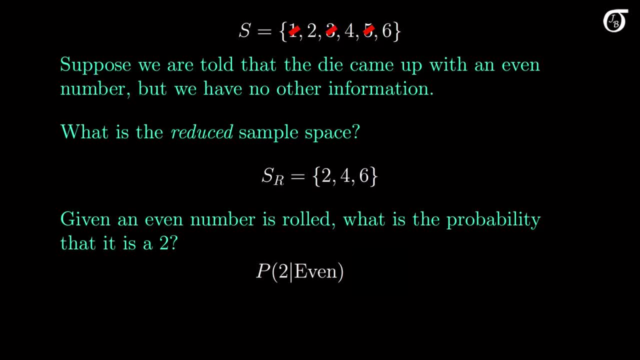 but let's first solve this using basic probability logic. The regular probability rules apply to the reduced sample space. Here we now have three remaining equally likely sample points. 2 is one of those three sample points. so the probability of getting a 2,- given we rolled an even number- is 1 out of 3.. 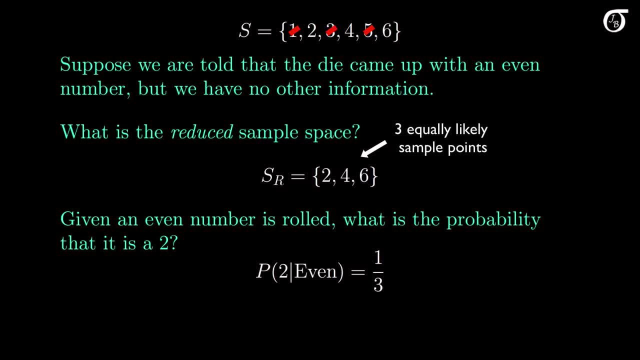 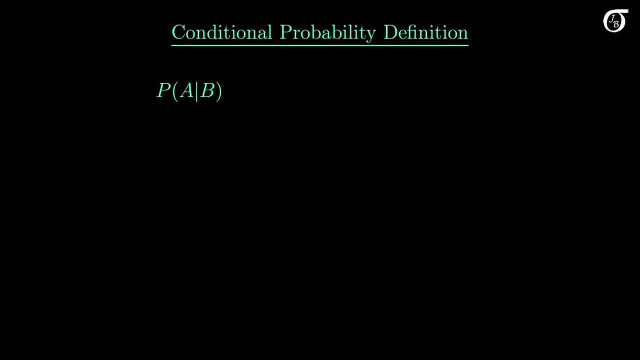 Knowing the number is even has doubled the probability that it is a 2.. Now that we've had a bit of motivation for it, let's look at the actual definition of conditional probability. We write the conditional probability of event A, given that event B has occurred, in this fashion. 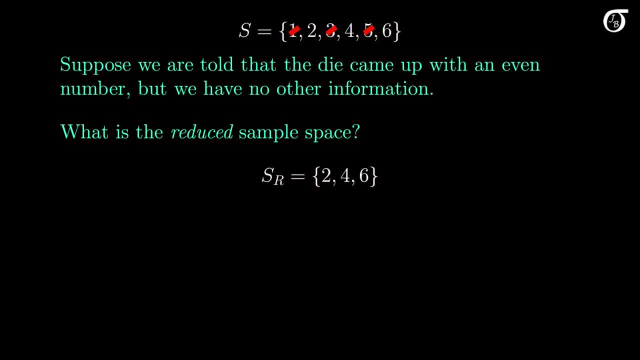 The reduced sample space is now the even numbers. Suppose we were asked the question: given an even number is rolled, what is the probability it is a 2? Here we are looking for a conditional probability, the probability that we rolled a 2, if we know the number is even. 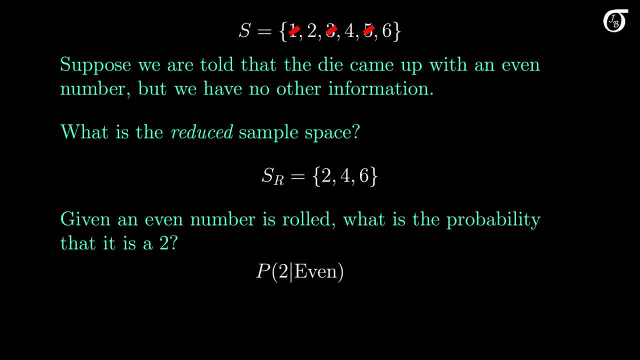 Notation-wise, we might write that as the probability of 2, given even where what comes after the vertical bar is known to be true or assumed to be true for the purposes of the question. Now, in a moment we are going to look at the official definition of conditional probability. 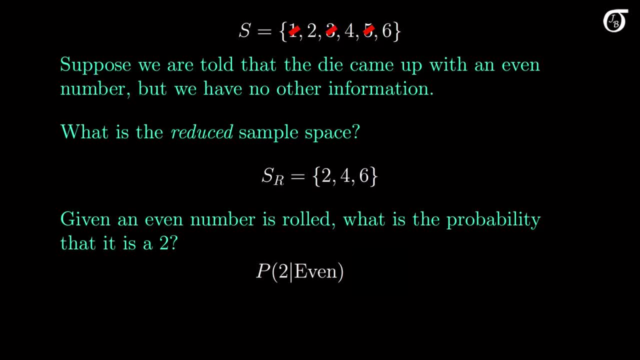 but let's first solve this using basic probability logic. The regular probability rules apply to the reduced sample space. Here we now have three remaining equally likely sample points. 2 is one of those three sample points. so the probability of getting a 2,- given we rolled an even number- is 1 out of 3.. 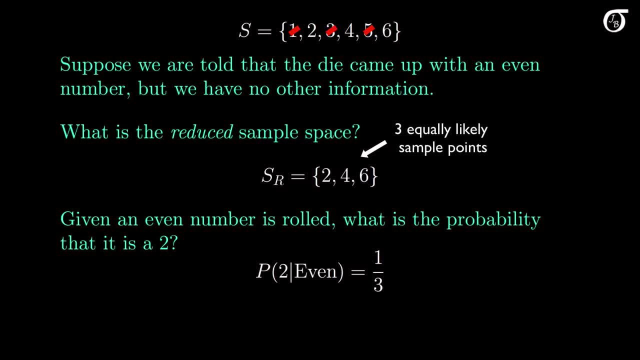 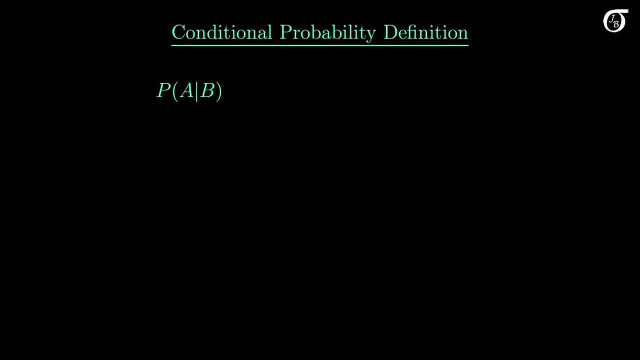 Knowing the number is even has doubled the probability that it is a 2.. Now that we've had a bit of motivation for it, let's look at the actual definition of conditional probability. We write the conditional probability of event A, given that event B has occurred, in this fashion. 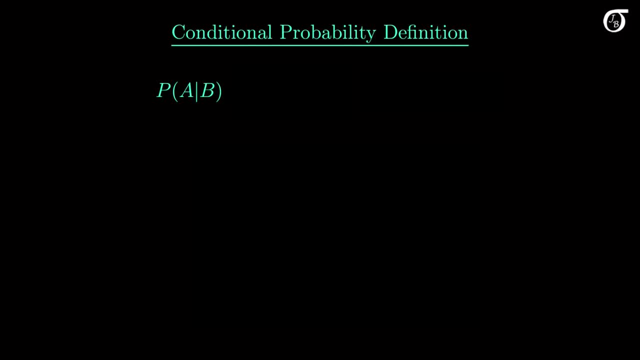 Again, anything to the right of the vertical bar is known to have occurred or assumed to have occurred. The conditional probability is defined to be the probability of the intersection of A and B over the probability of event B, The probability of the intersection over the probability of what we are taking as given. 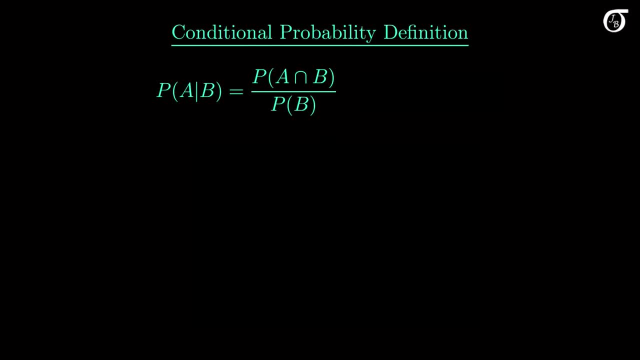 We do have one restriction we need to put in to shore this up mathematically. This formula won't work if the probability of event B is 0, since we were run into a 0 over 0 issue. So the conditional probability of event A given B is only defined if the probability of event B is greater than 0.. 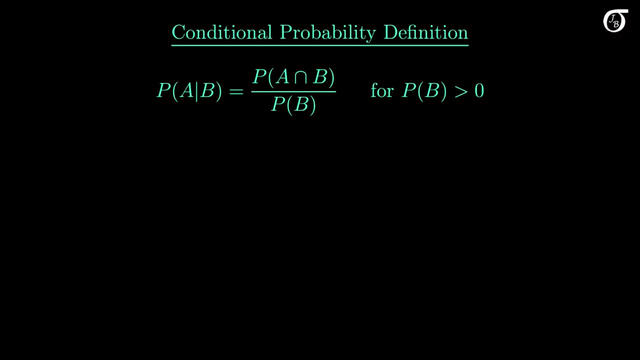 This isn't often a meaningful restriction in practice, as we aren't typically interested in conditioning on events that have no chance of occurring. So that's the definition of the conditional probability of event A given event B has occurred. But why is that the appropriate formula? 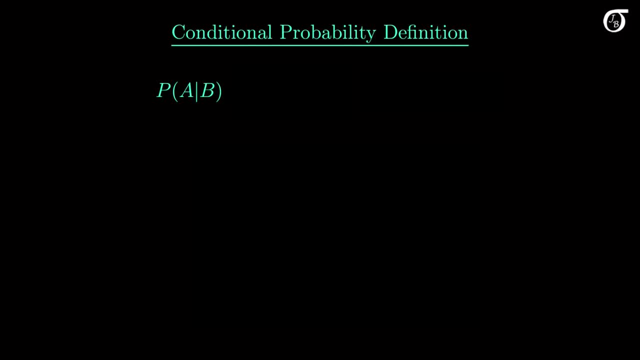 Again, anything to the right of the vertical bar is known to have occurred or assumed to have occurred. The conditional probability is defined to be the probability of the intersection of A and B over the probability of event B, The probability of the intersection over the probability of what we are taking as given. 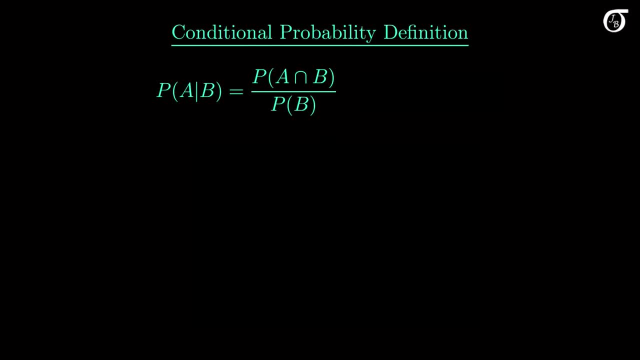 We do have one restriction we need to put in to shore this up mathematically. This formula won't work if the probability of event B is 0, since we were run into a 0 over 0 issue. So the conditional probability of event A given B is only defined if the probability of event B is greater than 0.. 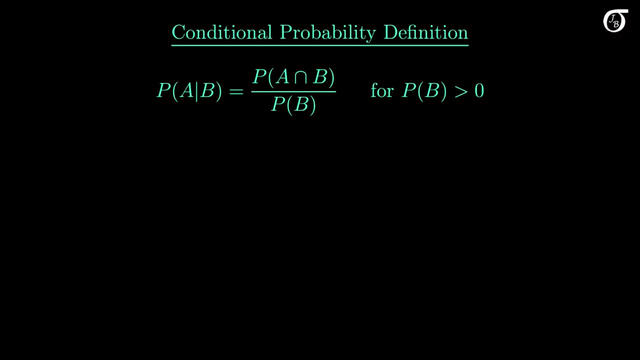 This isn't often a meaningful restriction in practice, as we aren't typically interested in conditioning on events that have no chance of occurring. So that's the definition of the conditional probability of event A given event B has occurred. But why is that the appropriate formula? 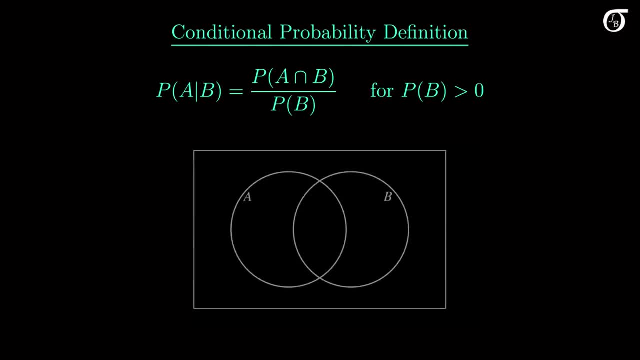 Why does that make sense? Here's a Venn diagram: representation of events A and B. The rectangle represents the entire sample space. Event A is represented by the circle on the left and event B by the circle on the right. Suppose we would like to know the probability of event A, given that event B has occurred. 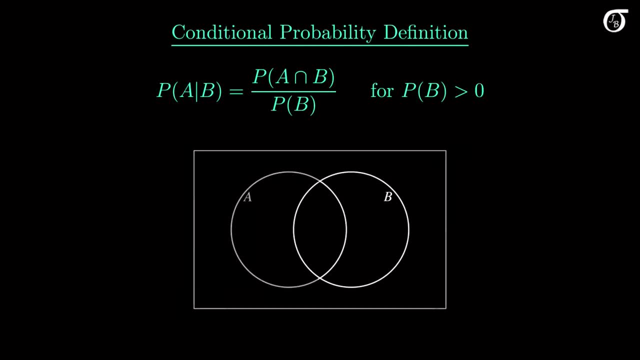 We are given B has occurred, so that reduces the sample space down to just event B, just the circle on the right. That is what our universe has been reduced to. If event B has occurred and we are in this circle, what is the probability that event A has also occurred? 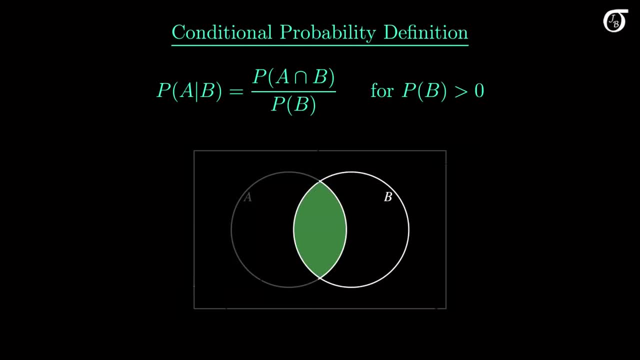 Event A shares this green region with event B. That's the AB intersection. So if we know that event B has occurred and we'd like to know the probability that A has also occurred, that will be the probability of the intersection of the two events. 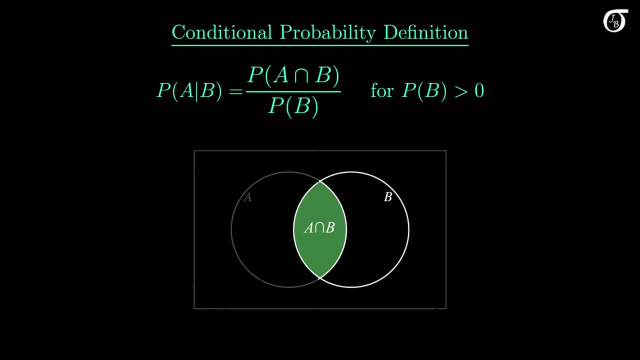 over the probability of event B, the reduced sample space. So the conditional probability definition is consistent with our intuitive notion of what a conditional probability should be. Please do me a small favor and don't try to memorize the definition of conditional probability. instead, try to understand the logic behind it. 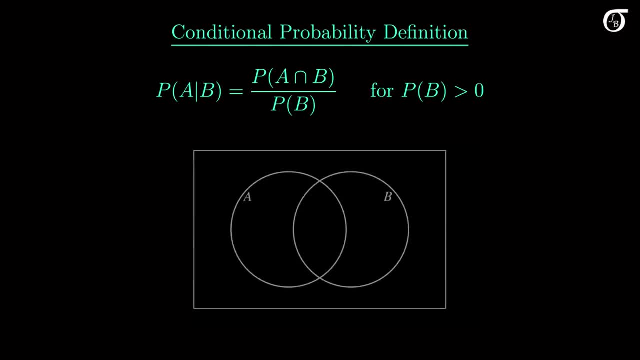 Why does that make sense? Here's a Venn diagram: representation of events A and B. The rectangle represents the entire sample space. Event A is represented by the circle on the left and event B by the circle on the right. Suppose we would like to know the probability of event A, given that event B has occurred. 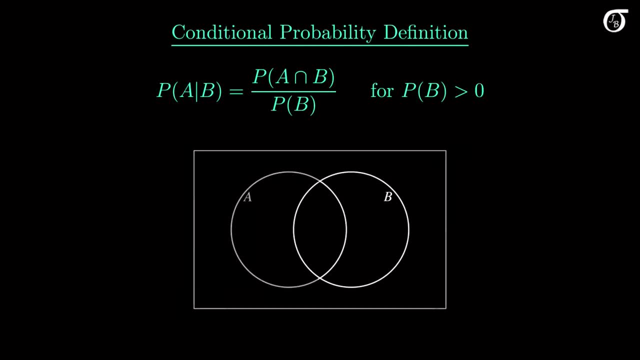 We are given B has occurred, so that reduces the sample space down to just event B, just the circle on the right. That is what our universe has been reduced to. If event B has occurred and we are in this circle, what is the probability that event A has also occurred? 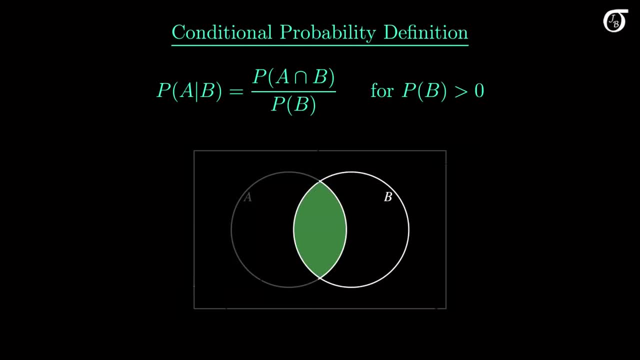 Event A shares this green region with event B. That's the AB intersection. So if we know that event B has occurred and we'd like to know the probability that A has also occurred, that will be the probability of the intersection of the two events. 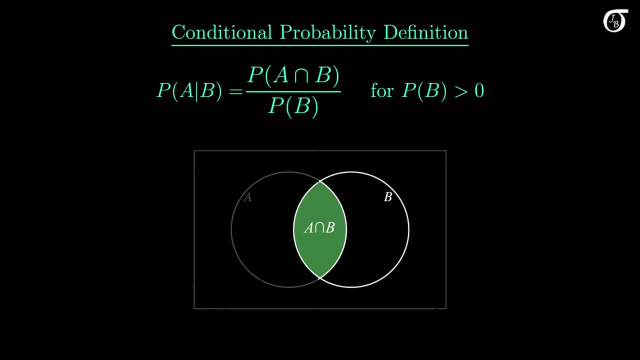 over the probability of event B, the reduced sample space. So the conditional probability definition is consistent with our intuitive notion of what a conditional probability should be. Please do me a small favor and don't try to memorize the definition of conditional probability. instead, try to understand the logic behind it. 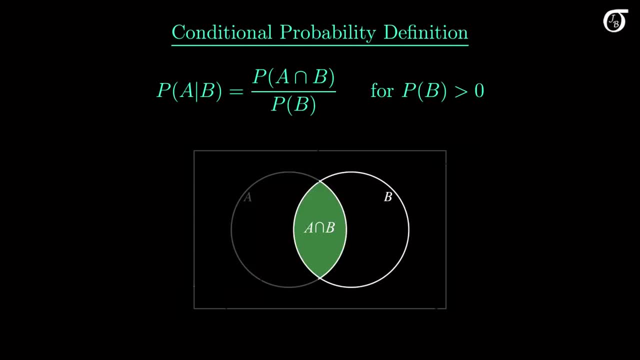 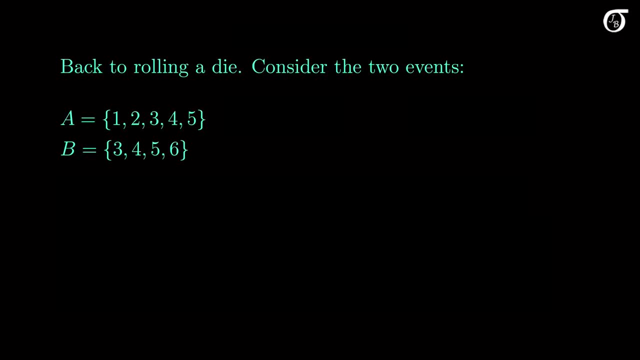 If you're able to do that, you'll never forget it. Let's work through a few examples. Back to die rolling and consider these two events. A: the event that we roll a 1,, 2,, 3,, 4, or 5,. 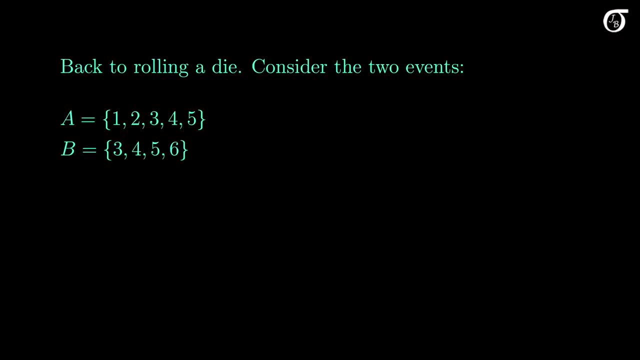 and B the event we roll a 3,, 4,, 5, or 6.. Recall that the sample space consists of these six equally likely numbers. What is the conditional probability of event A, given that event B has occurred? It's often easier to think logically through the problem. 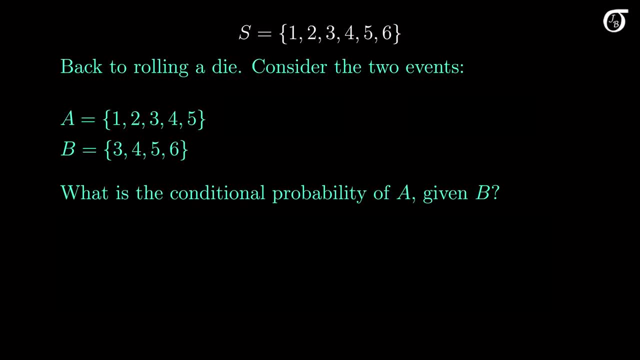 rather than jumping straight to the conditional probability formula. The formula always works if applied correctly, but it's often easier to simply think the problem through, So I'm going to do that here. then we'll work through the formula Here we are assuming event B has occurred. 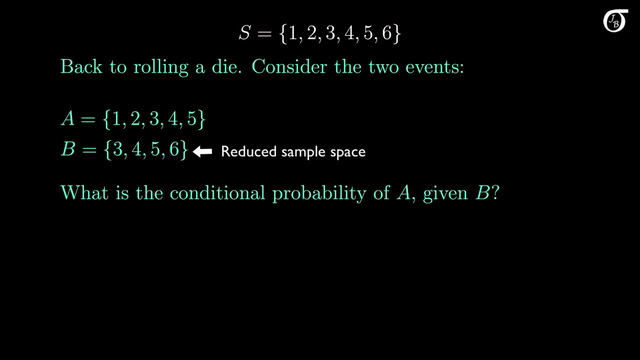 so the reduced sample space is event B, the numbers 3,, 4,, 5, and 6.. Within event B, the numbers 3, 4, and 5 are also part of A. the four sample points in B are all equally likely. 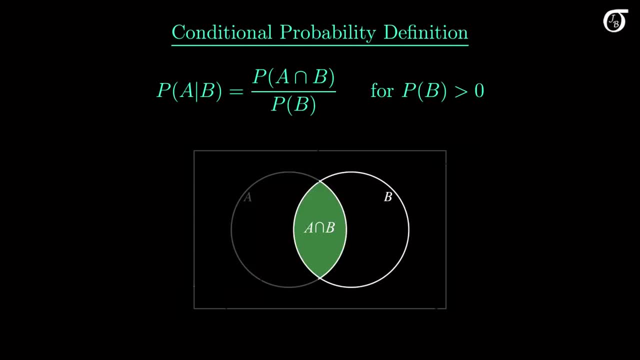 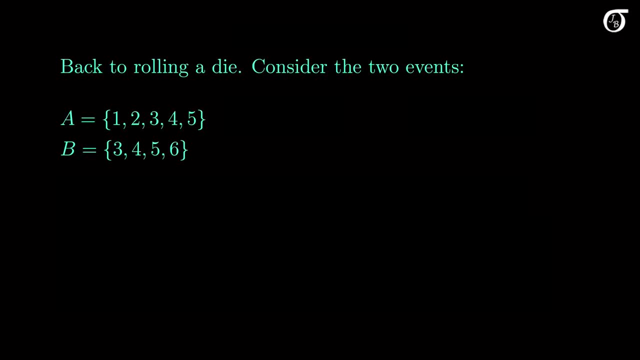 If you're able to do that, you'll never forget it. Let's work through a few examples. Back to die rolling and consider these two events. A: the event that we roll a 1,, 2,, 3,, 4, or 5,. 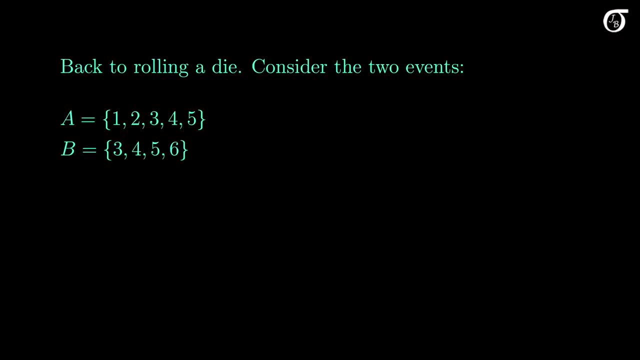 and B the event we roll a 3,, 4,, 5, or 6.. Recall that the sample space consists of these six equally likely numbers. What is the conditional probability of event A, given that event B has occurred? It's often easier to think logically through the problem. 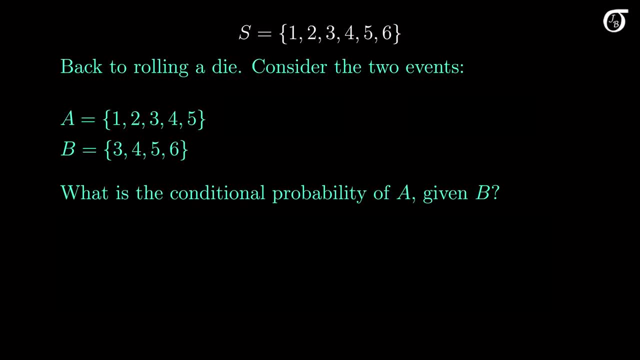 rather than jumping straight to the conditional probability formula. The formula always works if applied correctly, but it's often easier to simply think the problem through, So I'm going to do that here. then we'll work through the formula Here we are assuming event B has occurred. 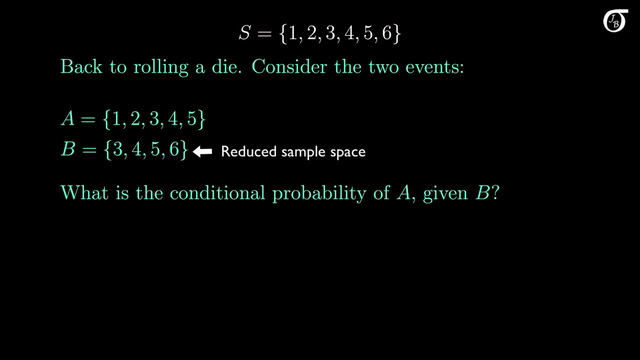 so the reduced sample space is event B, the numbers 3,, 4,, 5, and 6.. Within event B, the numbers 3, 4, and 5 are also part of A. the four sample points in B are all equally likely. 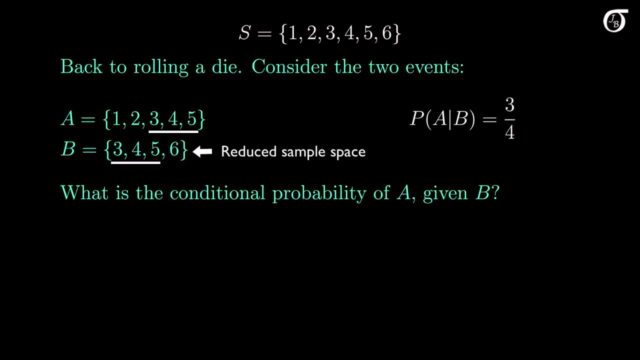 so the probability of event A given event B has occurred is 3 out of 4.. Working through the formula will yield the same probability, and let's see how that works. The conditional probability formula tells us that the conditional probability of A given B 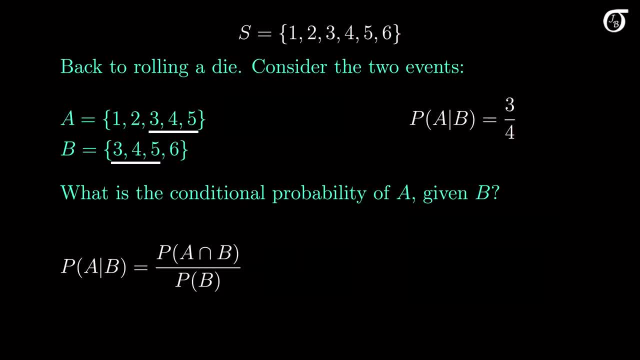 is the probability of their intersection over the probability of what we are given event B. The denominator is often straightforward to find. in this case, the probability of event B is simply 4 over 6, since we're dealing with equally likely sample points. 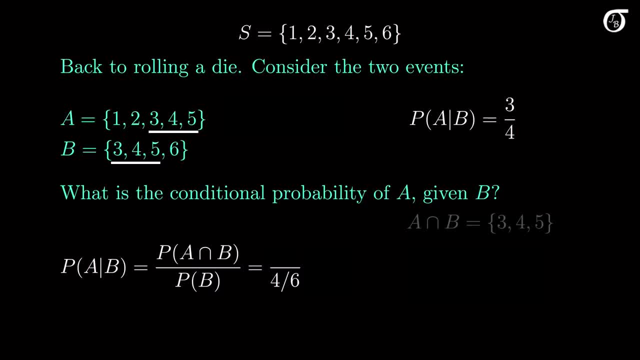 For the numerator A intersect B is the numbers 3,, 4, and 5,. since those occur in both A and B. The probability of the intersection is 3 out of 6, and thus the probability of A given B is 3 over 6 over 4 over 6,, which is 3 quarters. 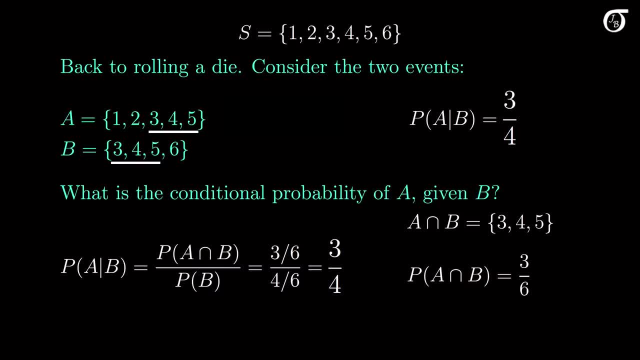 This is what we got above, using a little logic, Note that the unconditional probability of event A is 5 over 6,, since A contains 5 of the 6 equally likely sample points, The knowledge that event B has occurred, that the number is a 3,, 4,, 5, or 6,. 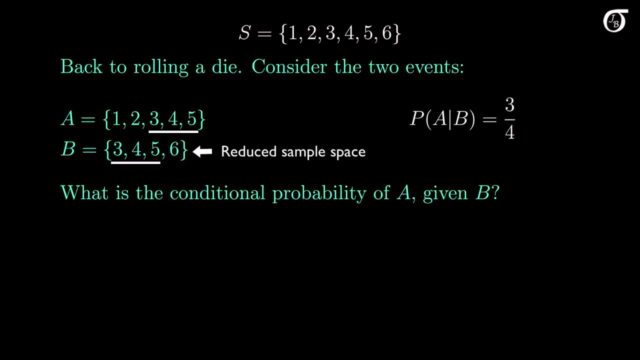 so the probability of event A given event B has occurred is 3 out of 4.. Working through the formula will yield the same probability, and let's see how that works. The conditional probability formula tells us that the conditional probability of A given B 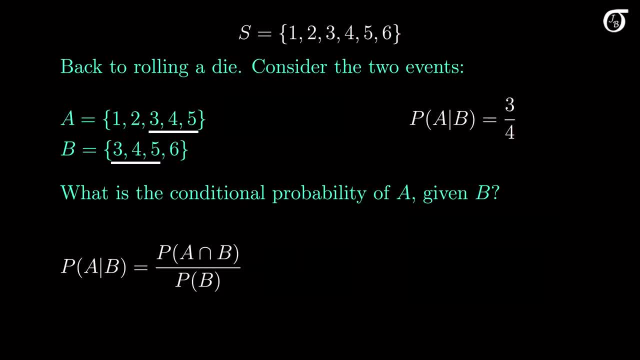 is the probability of their intersection over the probability of what we are given event B. The denominator is often straightforward to find. in this case, the probability of event B is simply 4 over 6, since we're dealing with equally likely sample points. 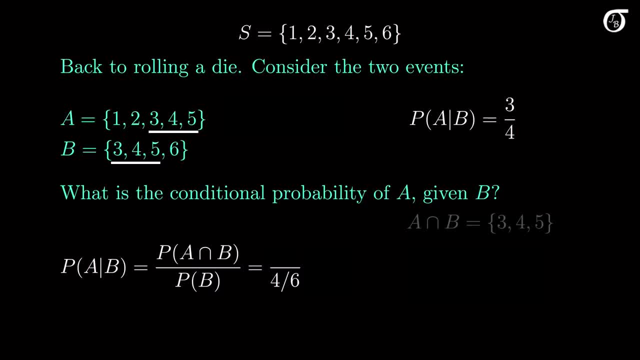 For the numerator A intersect B is the numbers 3,, 4, and 5,. since those occur in both A and B. The probability of the intersection is 3 out of 6, and thus the probability of A given B is 3 over 6 over 4 over 6,, which is 3 quarters. 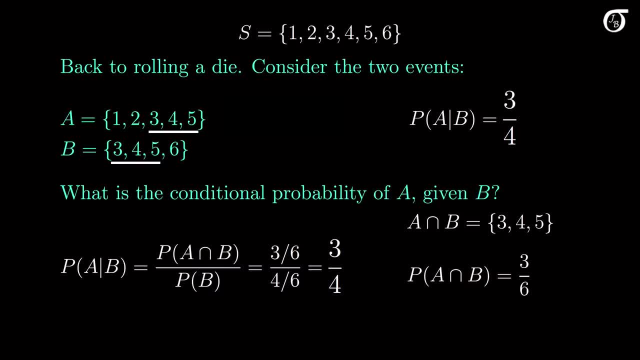 This is what we got above, using a little logic, Note that the unconditional probability of event A is 5 over 6,, since A contains 5 of the 6 equally likely sample points, The knowledge that event B has occurred, that the number is a 3,, 4,, 5, or 6,. 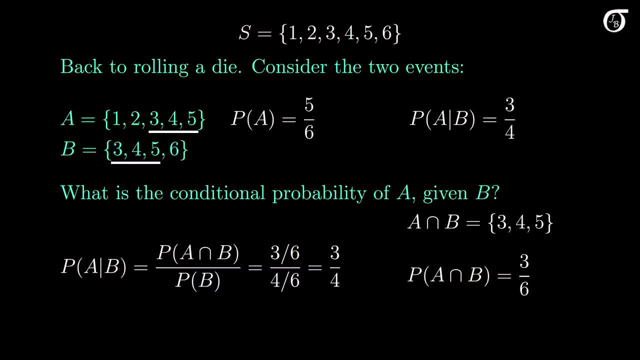 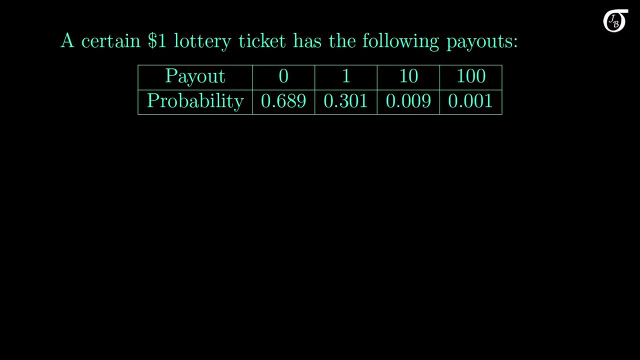 has reduced the probability of event A from 5 over 6 to 3 quarters. Now let's look at a simple example where the sample points are not equally likely. Suppose that a certain simple lottery has these payouts for a $1 ticket. 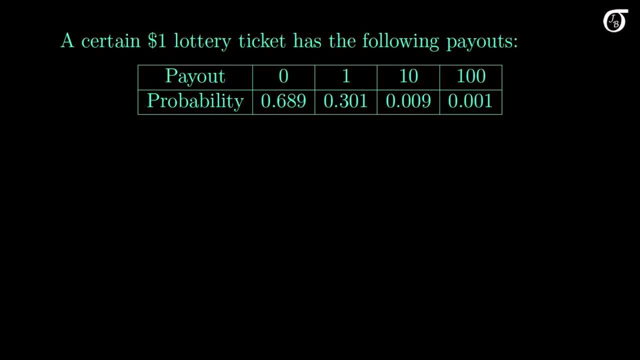 Most of the time we lose our money. sometimes we get our money back and occasionally we make a profit And suppose we're interested in this question. Given the payout is more than $1, what is the probability it is $10?? Before going to the formula, let's work through this one quickly. 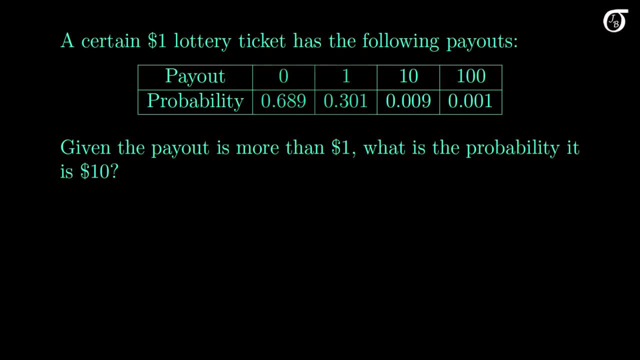 If we know the payout is more than $1, 0 or 1 can't have occurred, and that reduced our sample space down to these two possibilities. If it's one of these two possibilities, what is the probability it's $10?? 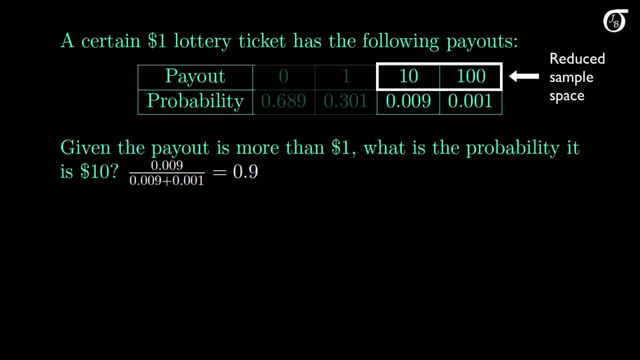 Just the probability of $10 over the sum of the two probabilities. So if we know the payout is greater than $1, there's a 90% chance it's $10.. Suppose we want to find this probability more formally using the formula: 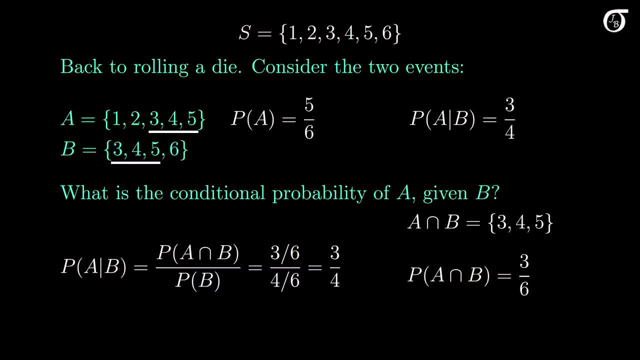 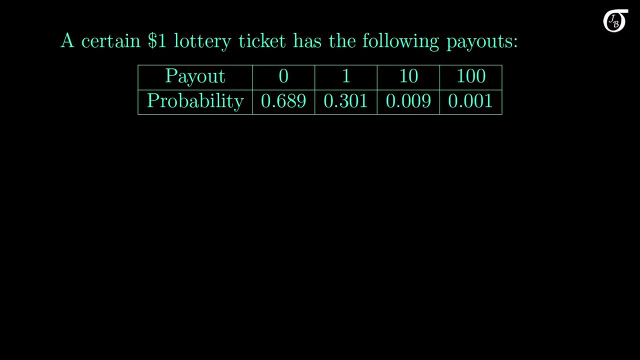 has reduced the probability of event A from 5 over 6 to 3 quarters. Now let's look at a simple example where the sample points are not equally likely. Suppose that a certain simple lottery has these payouts for a $1 ticket. 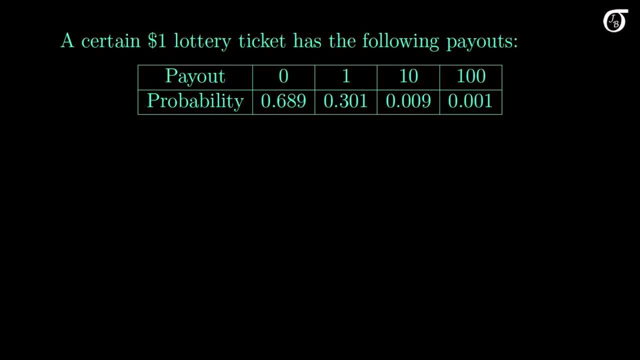 Most of the time we lose our money. sometimes we get our money back and occasionally we make a profit And suppose we're interested in this question. Given the payout is more than $1, what is the probability it is $10?? Before going to the formula, let's work through this one quickly. 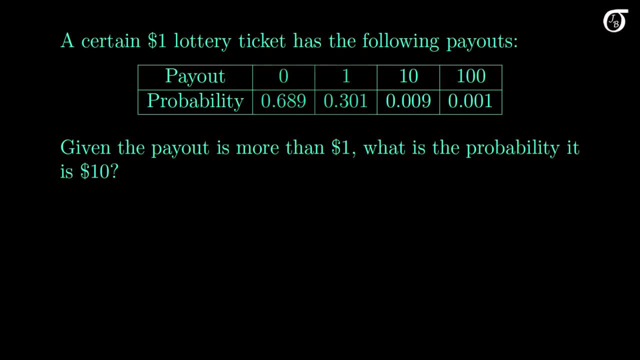 If we know the payout is more than $1, 0 or 1 can't have occurred, and that reduced our sample space down to these two possibilities. If it's one of these two possibilities, what is the probability it's $10?? 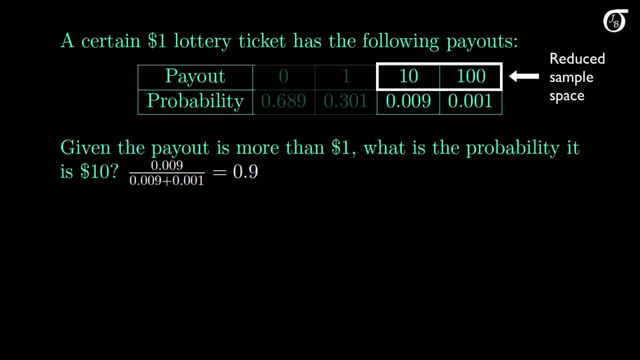 Just the probability of $10 over the sum of the two probabilities. So if we know the payout is greater than $1, there's a 90% chance it's $10.. Suppose we want to find this probability more formally using the formula: 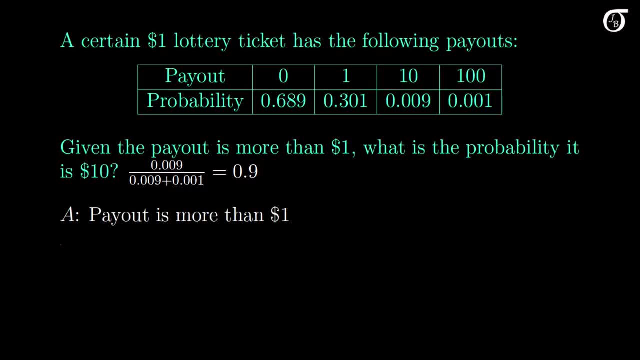 Let's define event A to be the payout being more than $1.. So A is made up of the events $10 and $100.. And the probability of A is 0.01.. The sum of the probabilities of $10 and $100. 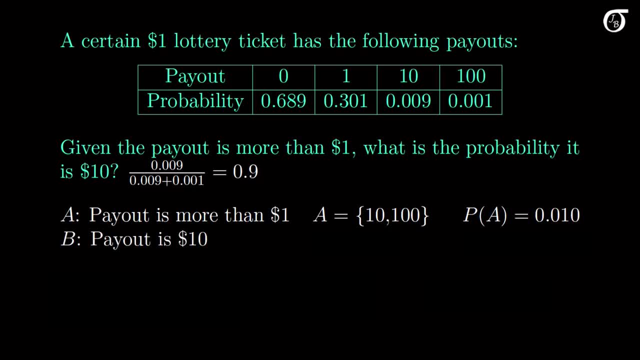 B is the event, the payout is $10.. So B is made up of just the number 10.. The probability of B is 0.009.. Here we want the probability. the payout is $10, given it's more than $1. 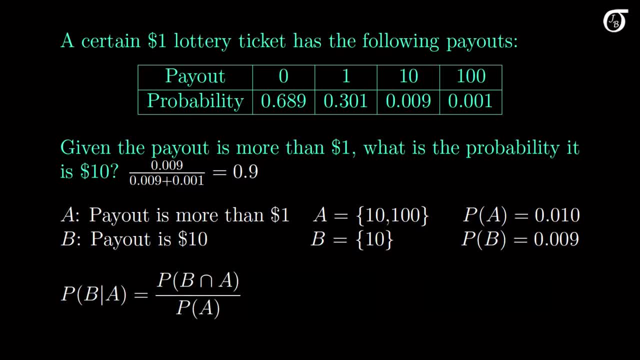 So we're looking for the probability of event B given A By the conditional probability formula, that's the probability of their intersection over the probability of what we are given event A. Where do these two events intersect? Only at 10,, since 10 is the only value that is contained in both A and B. 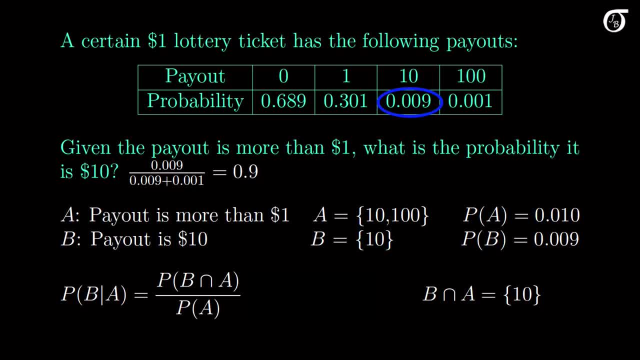 So the probability of their intersection is 0.009.. And the probability of event B, given A, is 0.009 over 0.01, or 0.9.. This is, of course, what we found above using a little logic. 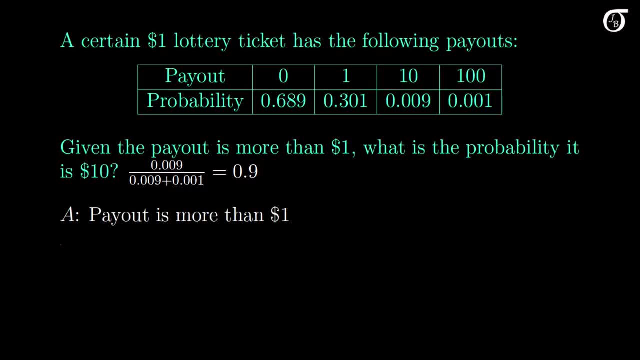 Let's define event A to be the payout being more than $1.. So A is made up of the events $10 and $100.. And the probability of A is 0.01.. The sum of the probabilities of $10 and $100. 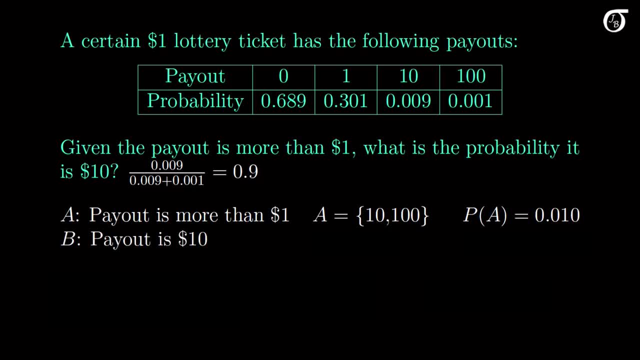 B is the event, the payout is $10.. So B is made up of just the number 10.. The probability of B is 0.009.. Here we want the probability. the payout is $10, given it's more than $1. 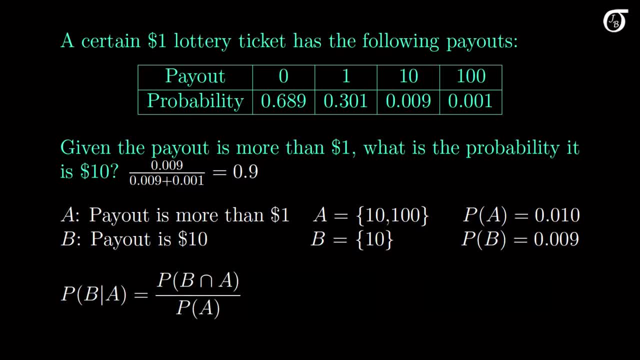 So we're looking for the probability of event B given A By the conditional probability formula, that's the probability of their intersection over the probability of what we are given event A. Where do these two events intersect? Only at 10,, since 10 is the only value that is contained in both A and B. 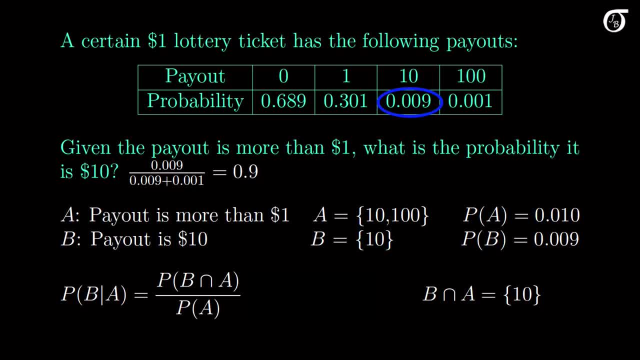 So the probability of their intersection is 0.009.. And the probability of event B, given A, is 0.009 over 0.01, or 0.9.. This is, of course, what we found above using a little logic. 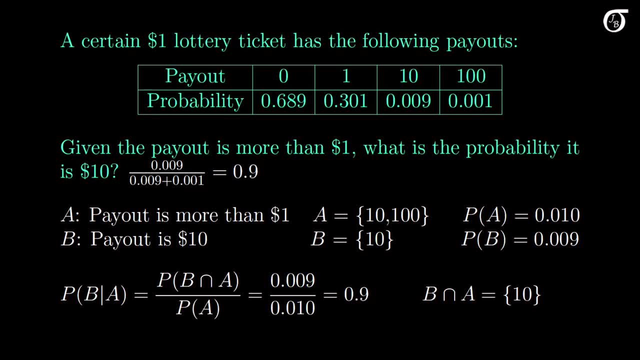 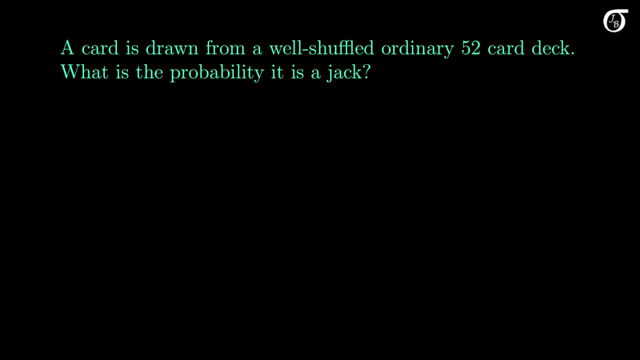 Now let's work through one more example, as I have one more point I'd like to make. Suppose a card is drawn from a well-shuffled, ordinary 52-card deck of playing cards And we'd like to know the probability it is a jack. 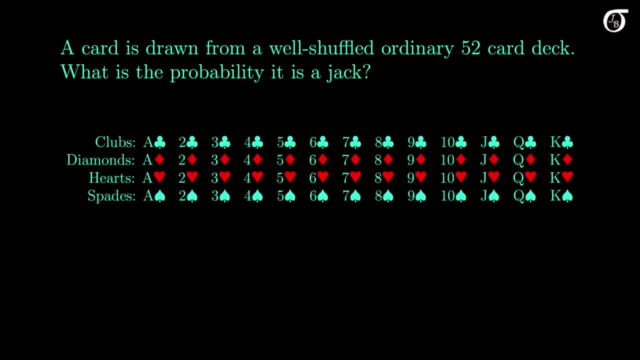 For those that don't know, a deck of 52 cards is made up of the ranks ace through king in each of four suits as illustrated here. Here we'll define our sample space to be these 52 cards. If it's a well-shuffled deck and everything's on the up and up. 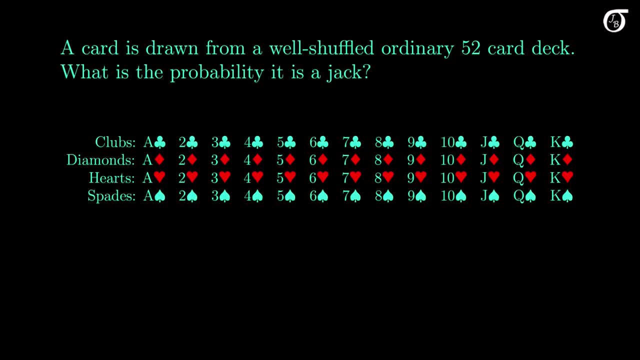 these 52 sample points will be equally likely. These four sample points are jacks, so the probability of drawing a jack is 4 out of 52, or 1 out of 13.. Now suppose we have extra information and we know the card is red. 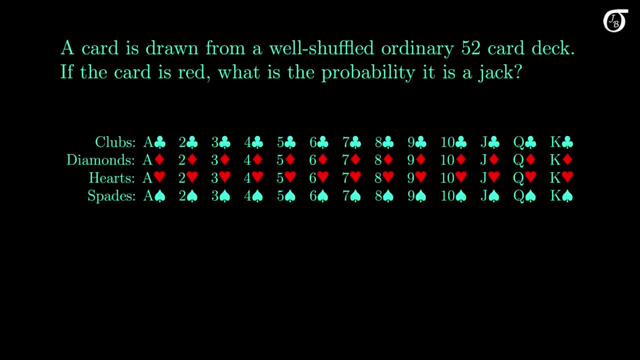 What is the probability? it is a jack, Although again, we could use the conditional probability formula to answer this question. this is a simple one that's a little easier to work through with the reduced sample space argument, So let's do that here. 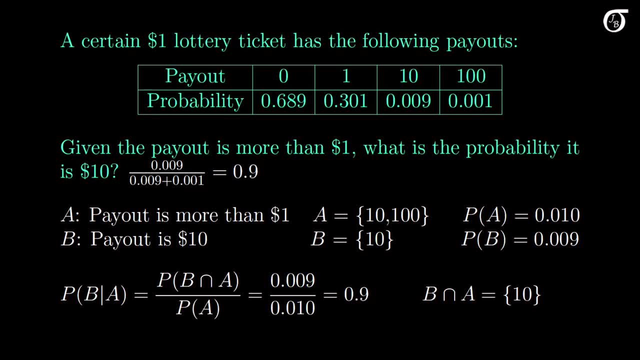 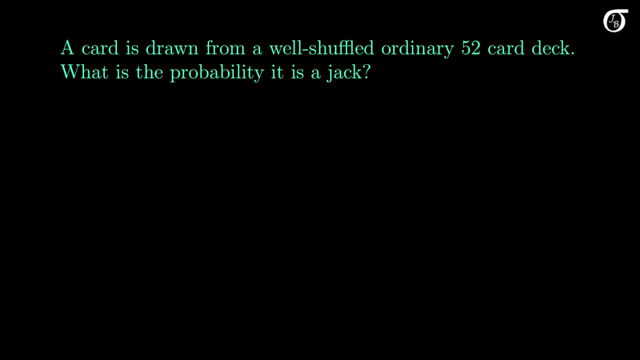 Now let's work through one more example, as I have one more point I'd like to make. Suppose a card is drawn from a well-shuffled, ordinary 52-card deck of playing cards And we'd like to know the probability it is a jack. 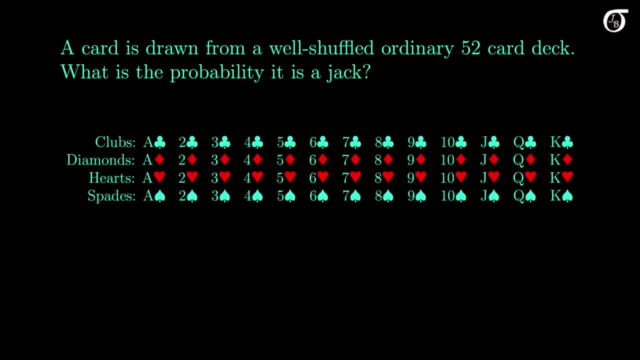 For those that don't know, a deck of 52 cards is made up of the ranks ace through king in each of four suits as illustrated here. Here we'll define our sample space to be these 52 cards. If it's a well-shuffled deck and everything's on the up and up. 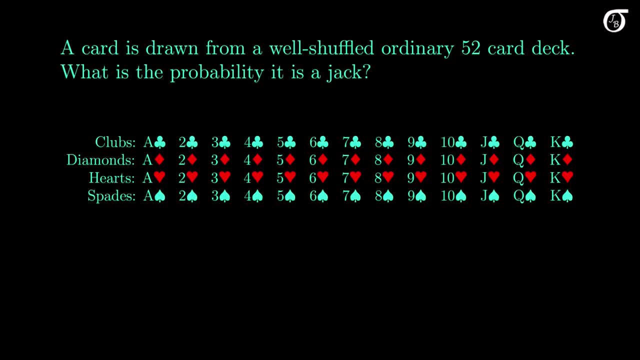 these 52 sample points will be equally likely. These four sample points are jacks, so the probability of drawing a jack is 4 out of 52, or 1 out of 13.. Now suppose we have extra information and we know the card is red. 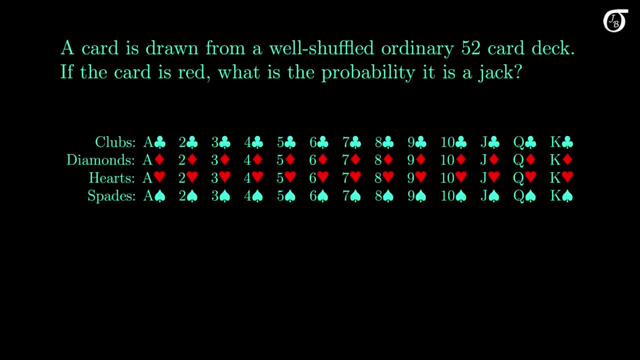 What is the probability? it is a jack, Although again, we could use the conditional probability formula to answer this question. this is a simple one that's a little easier to work through with the reduced sample space argument, So let's do that here. 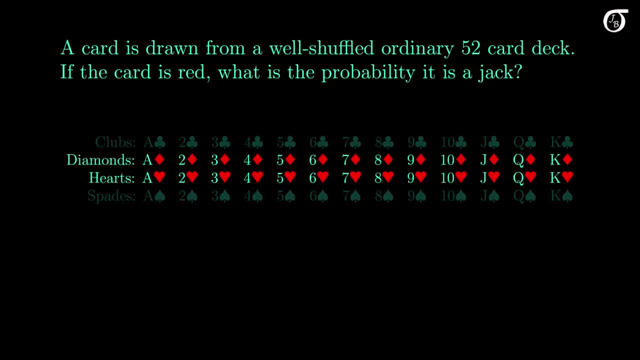 The knowledge that the card is red reduces the sample space down to just the red cards. Among these 26 equally likely red cards, two are jacks, and so the probability that the card is a jack, given it is red, is 2 out of 26, or 1 out of 13.. 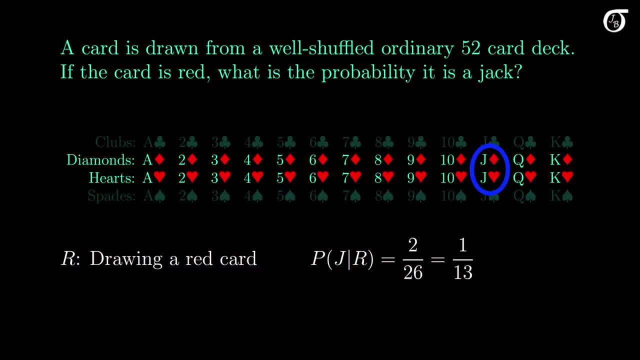 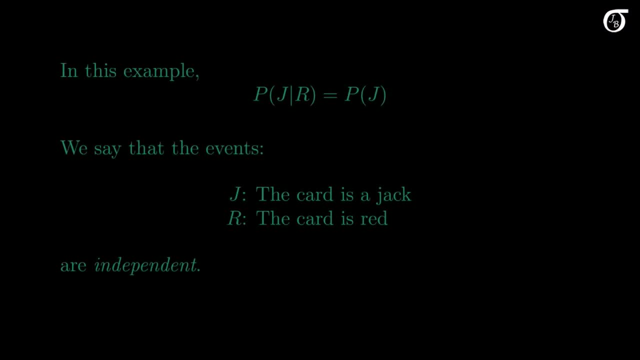 This is the same as the unconditional probability of drawing a jack that we found above, which leads to a very important point. In this example, the conditional probability the card is a jack, given it is red, is equal to the unconditional probability that the card is a jack. 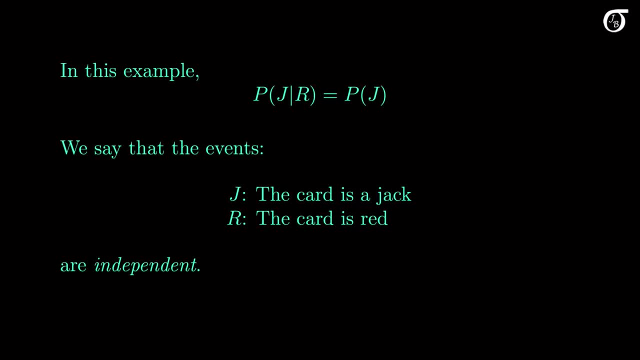 Because of this, we say that the two events are independent. Knowing that the card is red does not change the probability it is a jack. If we were betting on the card being a jack, we are indifferent to the information that the card is red. 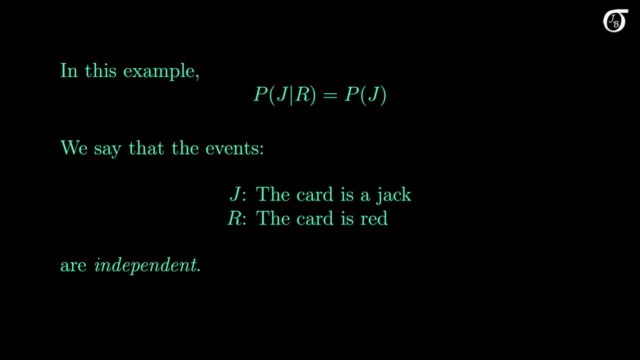 Independence is a very important concept in probability and statistics and I'll look at independence in much greater detail in another video. Conditional probability is an important concept as we often want to condition on information. We want to use all available information and use that information to properly adjust probabilities.